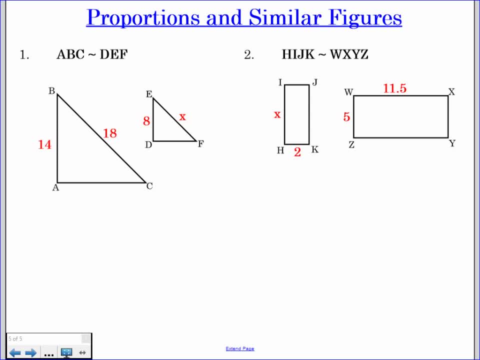 All right, we are going to look at proportions and similar figures, using proportions to find missing side lengths in similar figures. So we'll look at problem number one. here I have two triangles, ABC and DEF, and all I'm telling you here is the similarity statement saying that ABC. 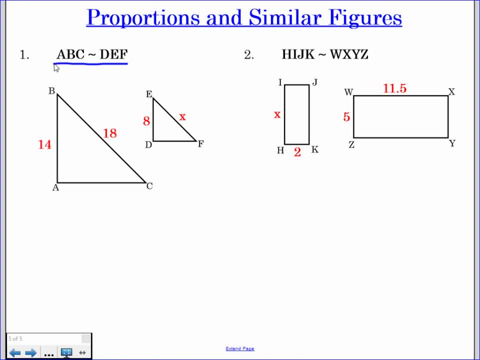 is similar to DEF. If I don't know that they're similar, then these problems aren't really solvable. I have to tell you that they're similar. Okay, so these two triangles are similar. Okay, in similar triangles, the ratios of corresponding sides are the same. So what that means is that. 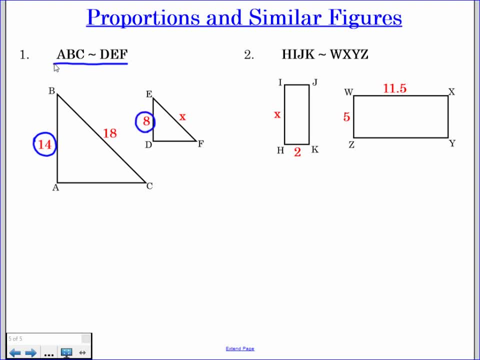 the ratio of 14 and its corresponding side of 8 has to be the same as the ratio of 18 and its corresponding side of x. Okay, so let's set up a proportion that says exactly that. Okay, let's say that 14 over x, or, I'm sorry, 14 over 8, equals 18 over x. That 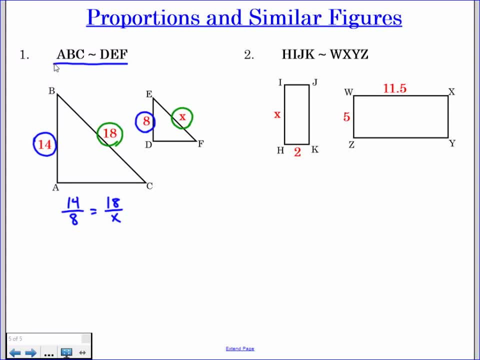 has to be true, And I'm going to solve this using cross products, just like I would any other proportion. So the cross products are going to say that 14 times x needs to be the same as 18 times 8. So that gives. 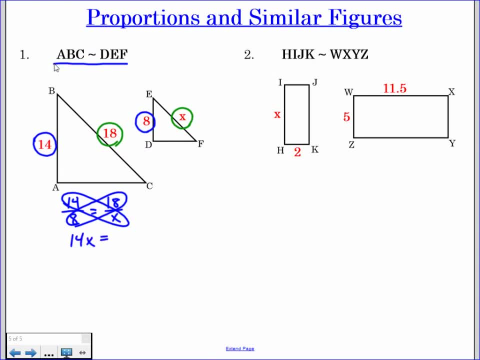 me the equation that says 14x is going to equal 18 times 8.. Let's go ahead and solve this. I'm going to leave the 14x alone for right now. 18 times 8 is 144.. I would divide by 14 to get x by. 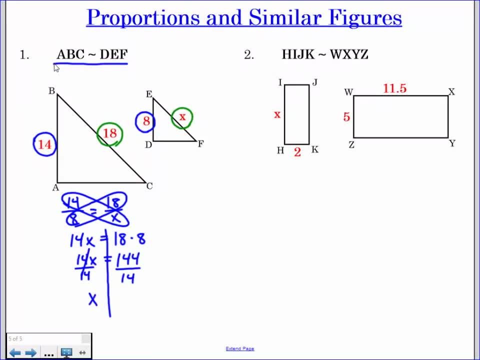 itself And that gives me a value for x. So our solution here is: x is about equal to 10.3.. Now, the only thing that I do want to make sure that we understand here: if I do 14 over 8, what I can't do is I can't do x over 18, because now 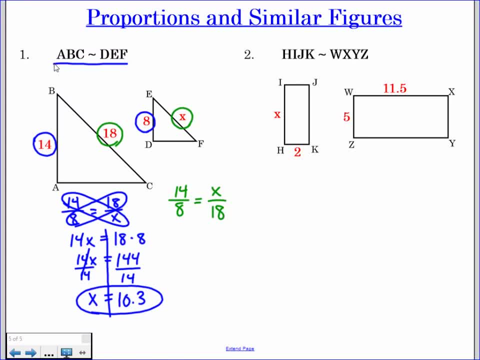 I'm changing the order of my ratios. Okay, I can't do that. Okay, if I do that, then that means I'm mixing up non-corresponding, Okay, so just be very careful. There's a lot of different ways to set up. 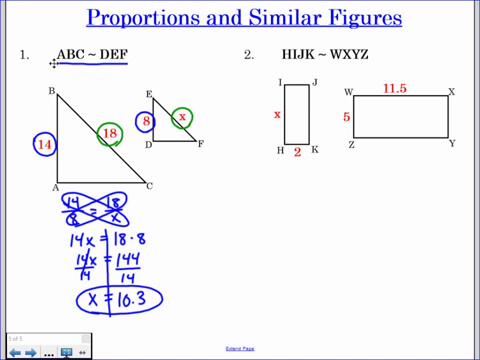 these proportions with these similar figures. Just make sure that you're keeping your order the same. However you do your first ratio, you have to follow that order for the second ratio. Next one, number two. Got two rectangles here. They are similar. I'm telling you that by giving 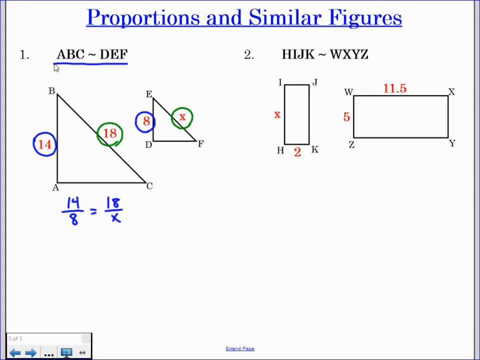 true. So let's set up a proportion that says exactly that. Okay, so let's set up a proportion, and I'm going to solve this using cross products, just like I would any other proportion. So the cross products are going to say that 14 times x needs to be the same as 18 times 8. So that gives. 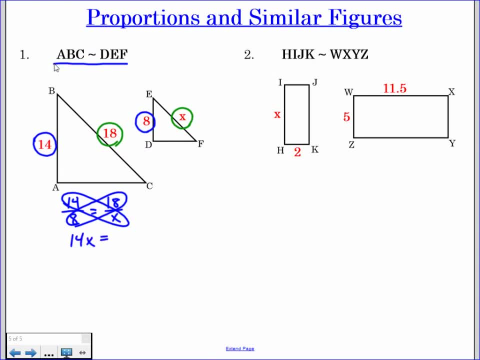 me the equation that says 14x is going to equal 18 times 8.. Let's go ahead and solve this. I'm going to leave the 14x alone for right now. 18 times 8 is 144.. I would divide by 14 to get x by. 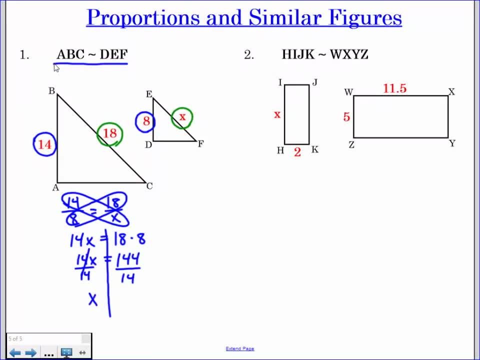 itself and that gives me a value for x. So our solution here is: x is about equal to 10.3.. Now, the only thing that I do want to make sure that we understand here: if I do 14 over 8, what I can't do is I can't do x over 18, because now 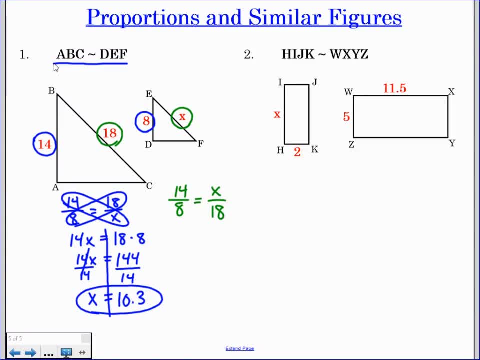 I'm changing the order of my ratios. I can't do that. If I do that, then that means I'm mixing up non-corresponding Okay. so just be very careful. There's a lot of different ways to set up these proportions with these similar figures. Just make sure that you're keeping your order. 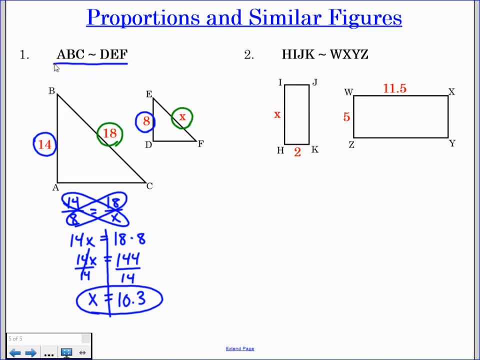 the same. However you do your first ratio, you have to follow that order for the second ratio. Next one, number two, Got two rectangles here. They are similar. I'm telling you that by giving you the similarity statement. Okay, so again, we have to be careful here, because the larger 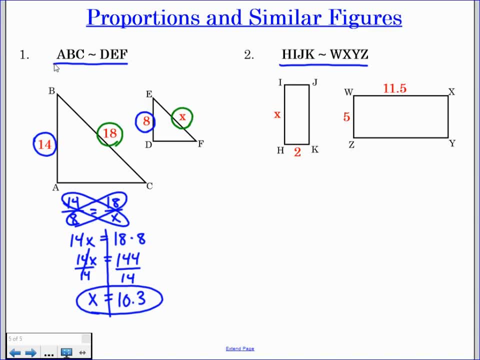 rectangle looks like it's rotated a little bit, So corresponding sides aren't going to line up quite as visually nice As problem number one. So you got to make sure that you catch here that two corresponds with five. Those are the two widths, the two short sides of our rectangles. 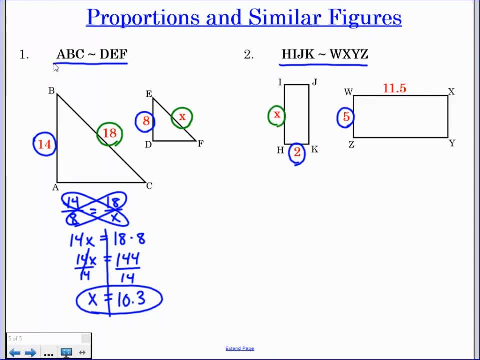 And then that means that x is going to correspond with 11.5.. So let's set up a proportion that says exactly that. So I'm going to say: okay, two over five needs to equal x over 11.5.. And again: 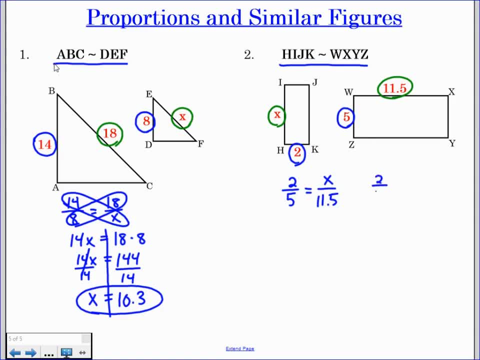 remember- just be careful with my order- What I cannot do. if I do two over five, I cannot do x over 11.5.. So I'm going to set up a proportion that says exactly that. So I'm going to say okay.